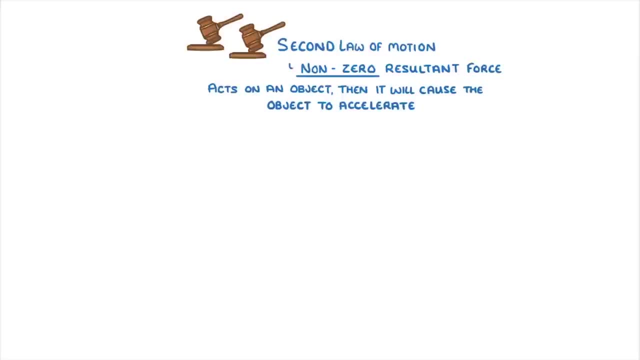 And remember, non-zero just means anything other than zero. For example, if we took this particle and we drew some unbalanced force arrows on it, we can see that there would be a resultant force to the right because the right arrow was bigger than the left arrow. 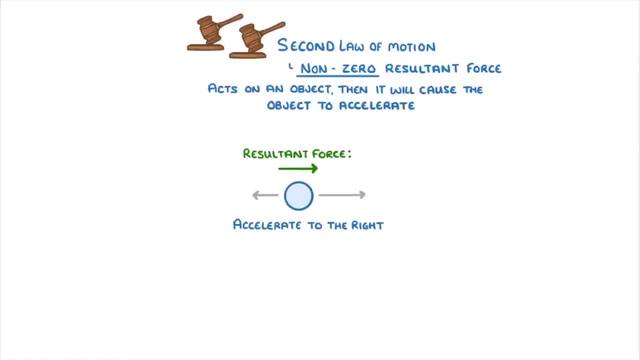 So this particle would accelerate to the right. Now, the confusing bit here is that, depending on the initial motion of the particle, this acceleration to the right could result in five different things happening. For example, if the object started off stationary, then the acceleration would cause it to start moving to the right. 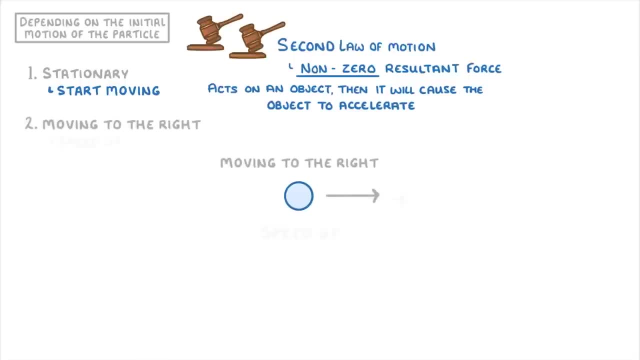 And if the object was already moving to the right, then it would cause it to speed up. However, if the object had been travelling to the left, then the rightwards acceleration would cause it to slow down, because it's acting in the opposite direction. 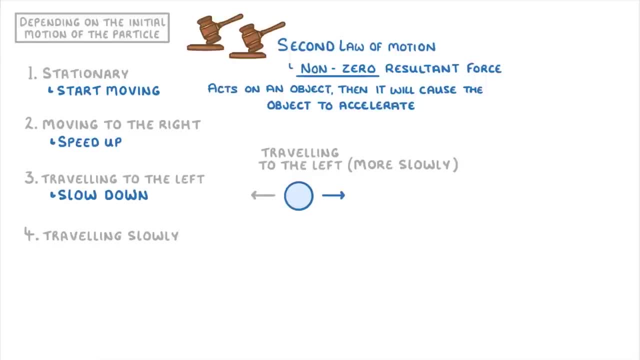 And if the object was travelling to the left more slowly, it could cause it to stop moving entirely because it was slowed down so much. The trickiest one to understand is that the acceleration could just result in a change in direction without any change in speed. 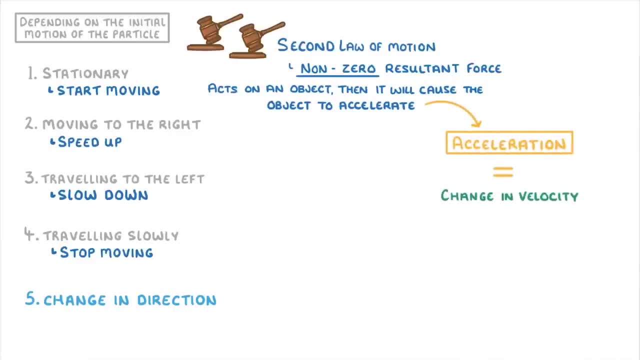 This is because acceleration is defined as the change in velocity divided by the change in time, And as velocity is determined by speed and direction, any change in the direction of the object also changes the velocity, and so is considered acceleration. We can see this in practice if we look at circular motion. 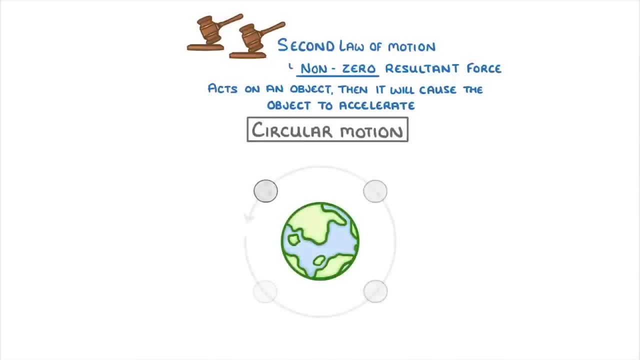 like the orbit of the moon around the earth. Even though the speed of the moon remains constant, we still say that it's accelerating because its direction is always changing slightly. This happens because the earth's mass exerts a gravitational pull on the moon. 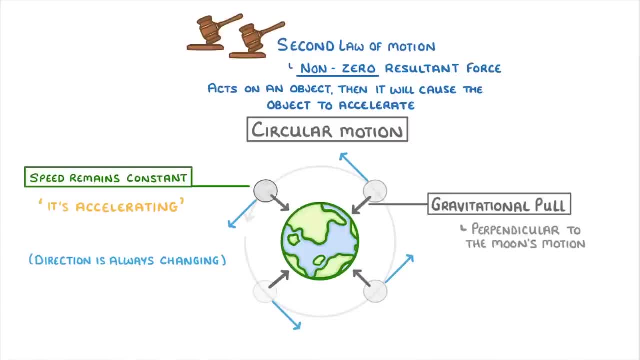 which acts perpendicular to the moon's motion. So overall, the moon ends up spinning around the earth with a constantly changing velocity, because the direction is changing, but a constant speed. The other part of Newton's second law is that the size of the resultant force 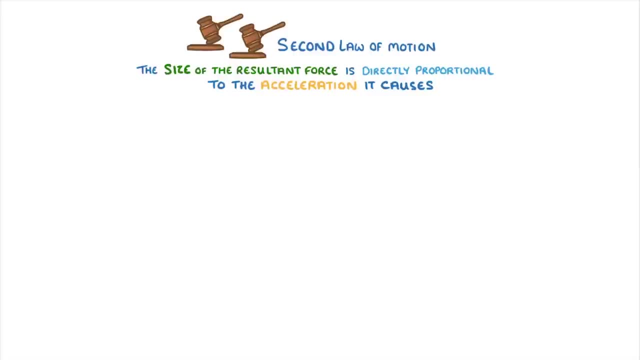 is directly proportional to the acceleration that it causes. For example, if you made the resultant force twice as big, then the acceleration that it causes would also be twice as big. We can see this in the equation F equals ma, which says that the resultant force is equal. 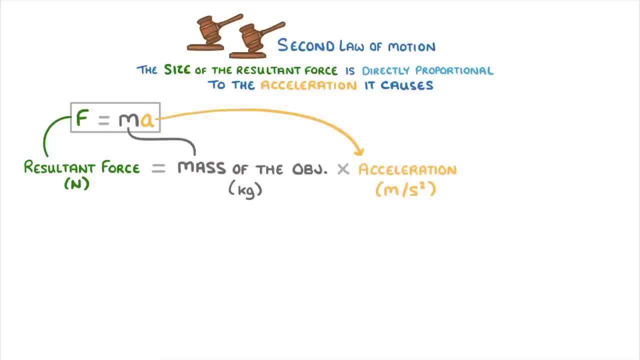 to the mass of the object multiplied by the acceleration that it causes. So if our particle from earlier had a mass of 0.25 kilos and was acted on by a force to the left of 30 newtons and a force to the right of 42 newtons, then we could use this information to work out its acceleration. 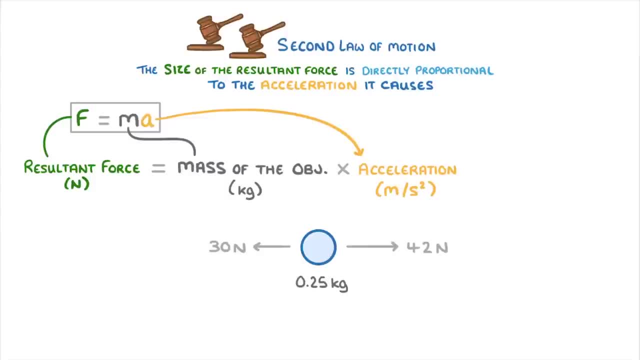 First we'd need to find the resultant force, which would be 42 minus 30, so 12 newtons to the right. Then we'd rearrange our equation to get force over mass equals acceleration and plug in our values to give 12 newtons over 0.25 kilos to get an acceleration of 48 m per second squared. 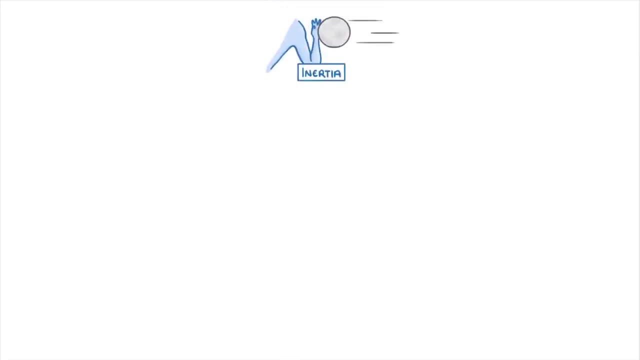 The last thing we need to cover is the idea of inertia, which is the tendency for the motion of an object to remain constant. The last thing we need to cover is the idea of inertia, which is the tendency for the motion of an object to remain constant. 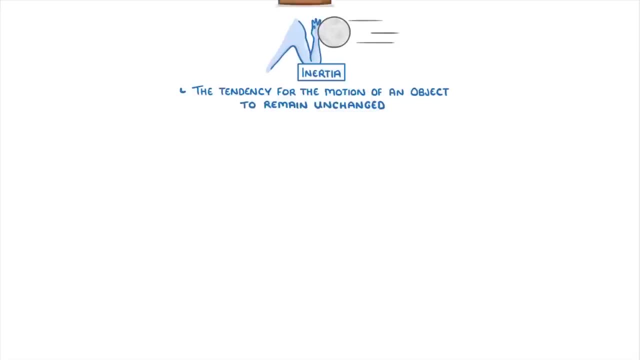 to remain unchanged. It's basically just Newton's first law, namely that unless acted on by resultant force, objects at rest will stay at rest and objects in motion will stay in motion. Meanwhile an object's inertial mass measures how difficult it is to change an object's velocity. 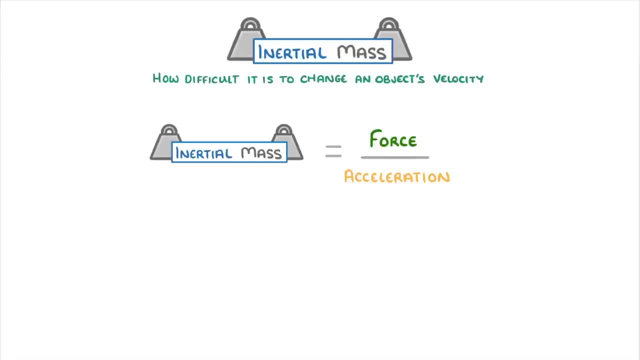 and we find it by dividing force, by acceleration, which is just the equation from Newton's second law again. So basically, a large mass like the moon will have a lot of inertia, so will require a really big force to change its velocity. 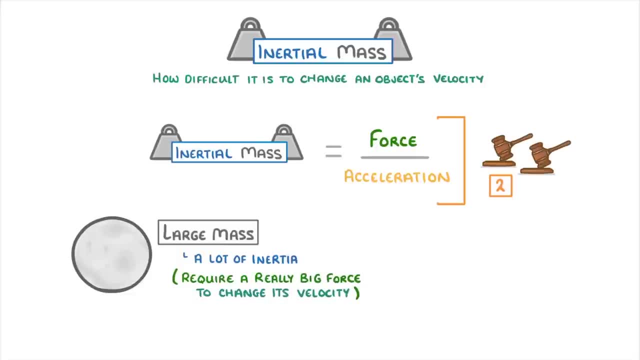 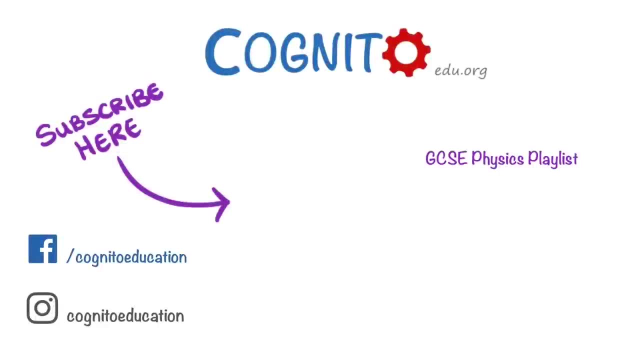 And even then the acceleration will probably be quite small. Anyway, that's everything for this video, So if you enjoyed it, then try checking out some of our other physics videos, and we'll see you next time.